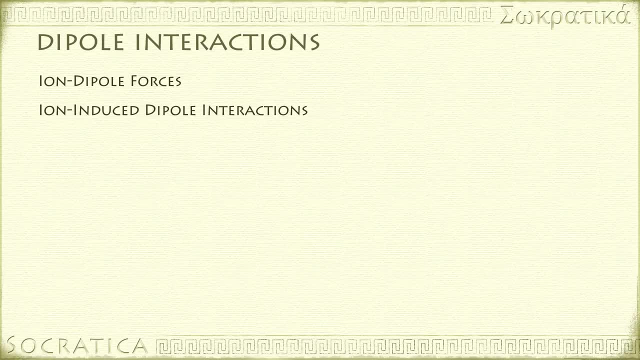 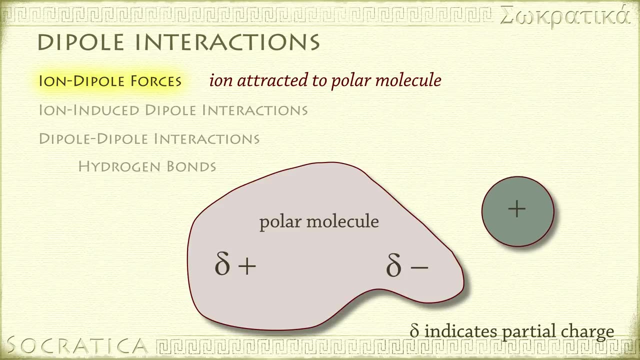 the various kinds of dipole interactions. Ion-dipole forces occur when ions are attracted to a polar molecule. positive ions are attracted to the negative end of a polar molecule and negative ions are attracted to the positive end, For example, when NaCl is in solution in water. 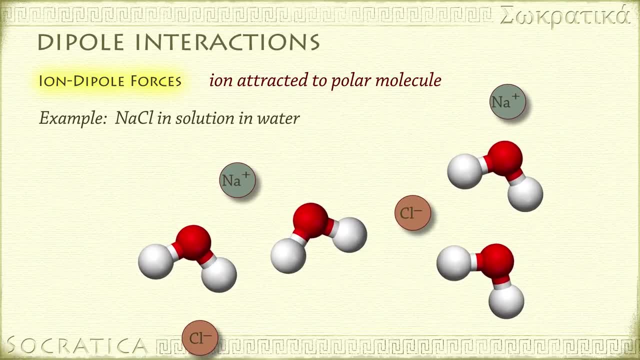 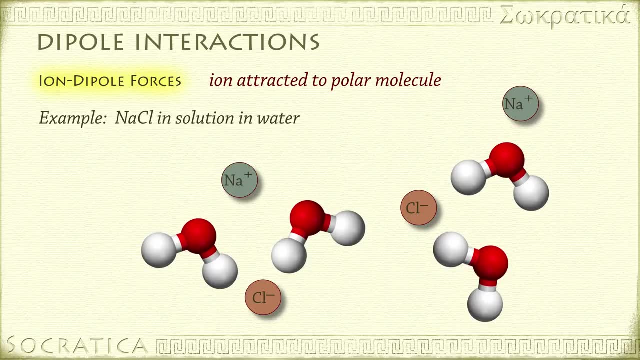 the negative end of NaCl is attracted to the positive end of NaCl. The positive end of the polar water molecules are attracted to the positive Na plus ions. So you can see the water molecules are oriented. so the oxygens with their partial negative 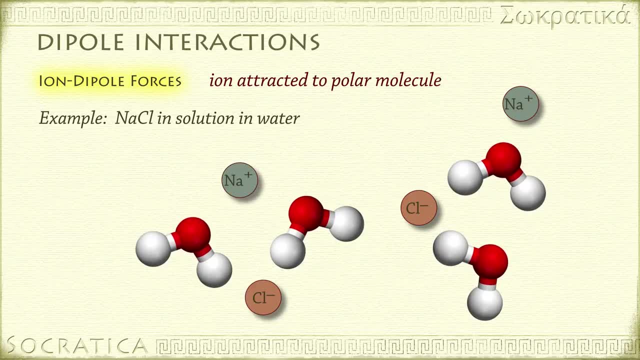 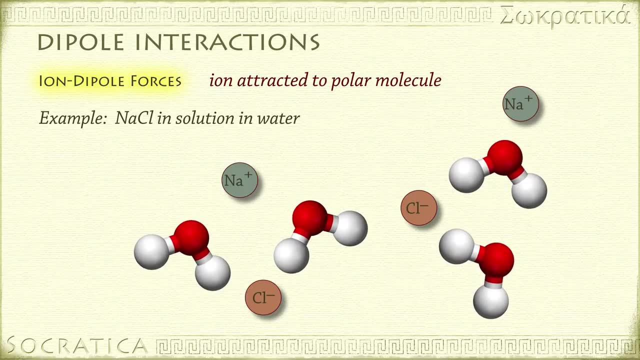 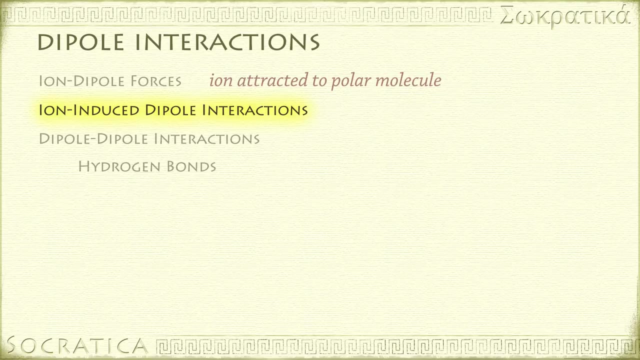 charges are pointed towards the Na plus ions and the hydrogens are pointed away. Meanwhile, the positive end of the water molecule is oriented towards the negative chloride ion. There are also cases of ion-induced dipole interactions. This is when the presence of the ion induces a temporary dipole in another molecule that usually 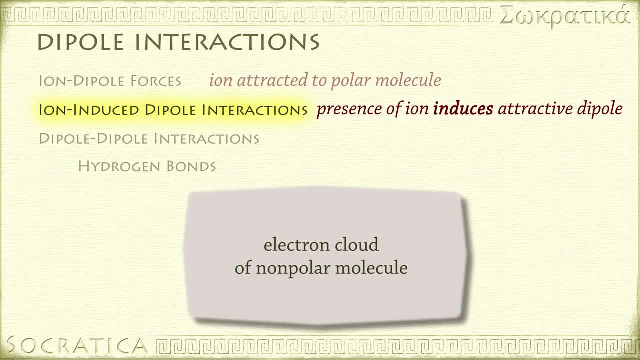 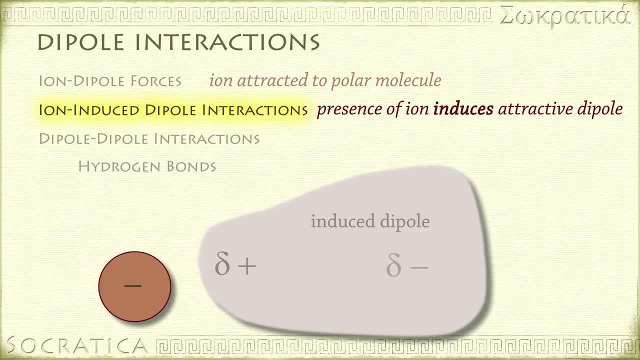 does not have poles. It's sitting there, being nonpolar, no partial positive or negative charges, until an ion approaches. The charge of the ion causes a temporary distortion of the electron cloud of the nonpolar molecule, inducing a dipole which is then attracted to the ion, For example. 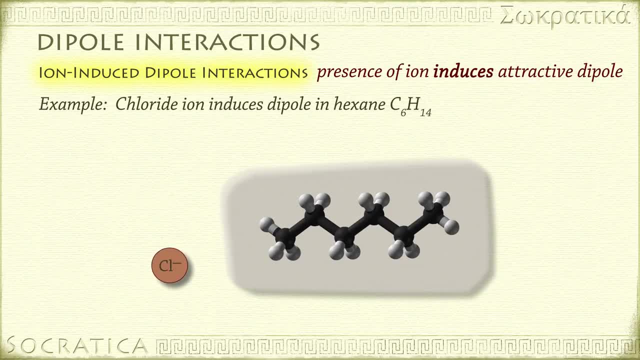 As this chloride ion Cl- approaches hexane C6H14, a non-polar molecule, the negative charge on the ion slightly distorts the electron cloud. It pushes the electrons away just a little. As a result, there is a slight partial positive charge on this side of the hexane. 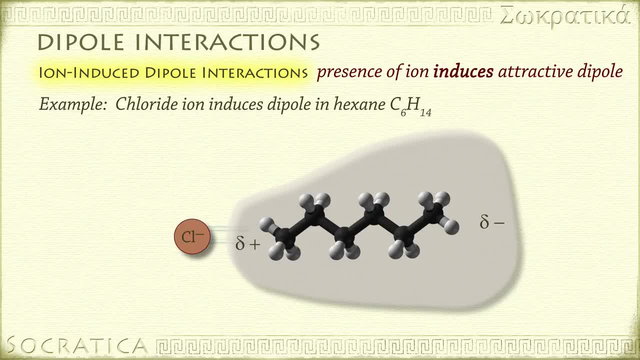 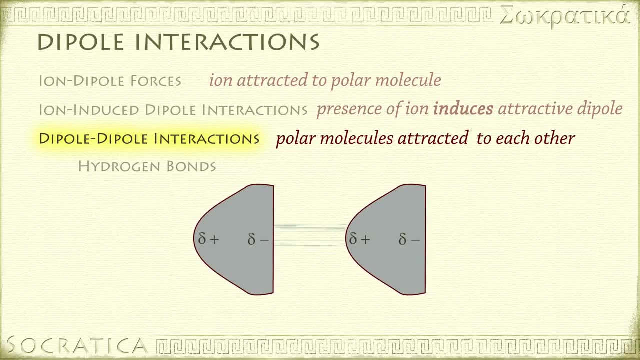 which is then attracted to the negatively charged ion. Dipole-dipole interactions occur when two polar molecules are very close to each other and the positive end of one polar molecule is near the negative end of the other molecule. The strength of the attraction increases with. 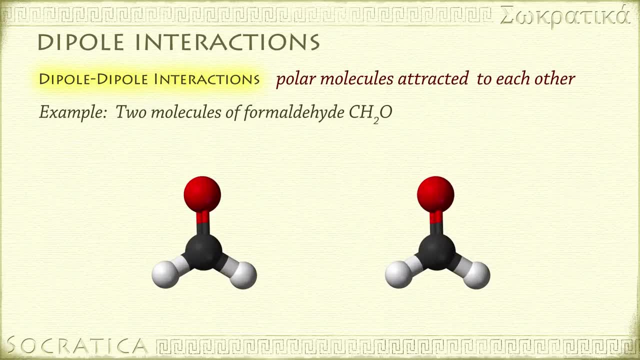 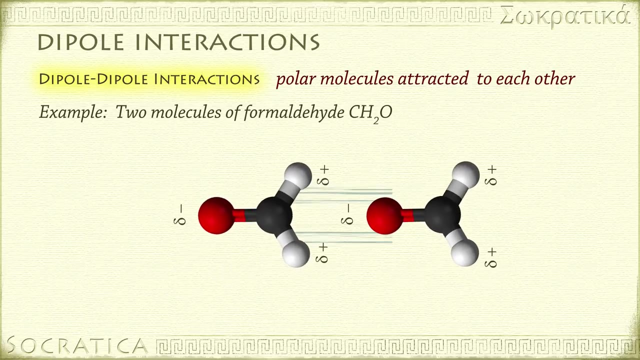 increasing polarity. Here, for example, you can see two molecules of formaldehyde, CH2O. Each of these individual molecules contains a polar covalent bond. The molecules have positive and negative ends, or poles. If two formaldehyde molecules come close together, 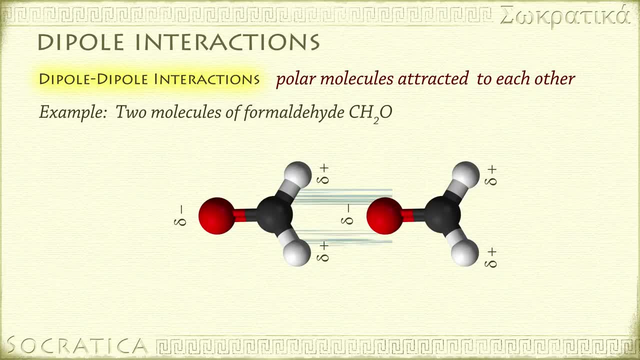 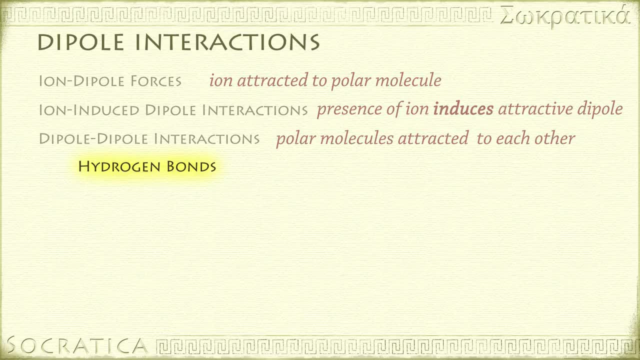 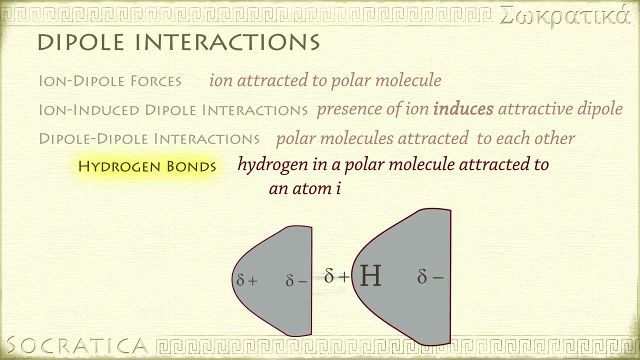 the partial positive end of one molecule will be attracted to the partial negative end of the other molecule. A special case of dipole-dipole interaction is the hydrogen bond. This is when the hydrogen atom in a very polar molecule is attracted to the negatively charged. 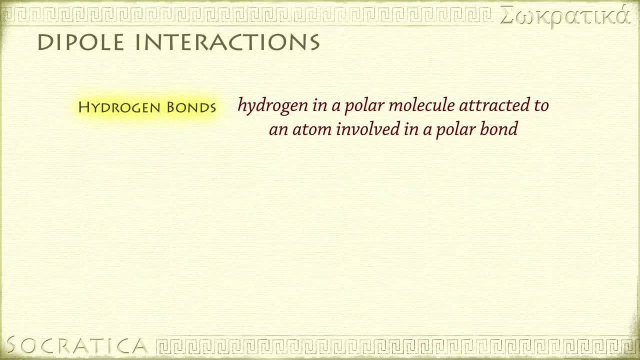 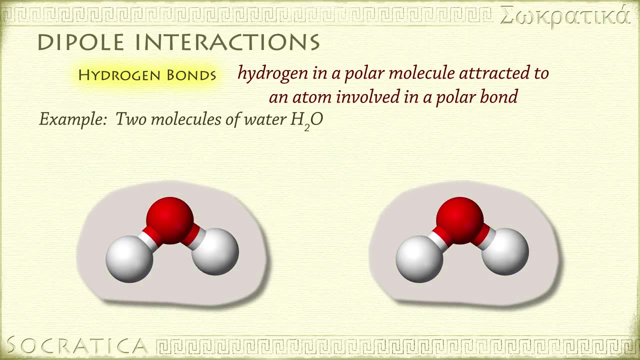 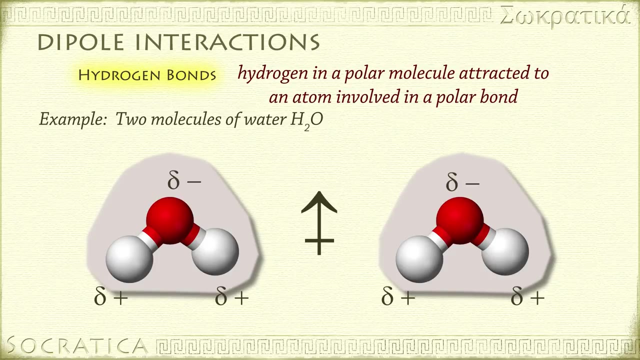 atom in another polar molecule. The hydrogen is most often involved in a bond with a fluorine oxygen or nitrogen. Fluorine oxygen and nitrogen are so electronegative they are typically involved in extremely polar bonds. These electronegative atoms pull electrons. 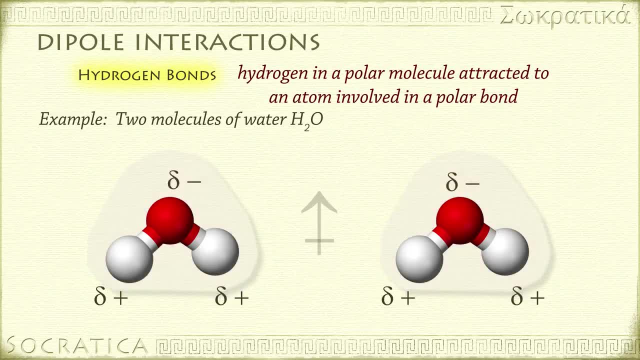 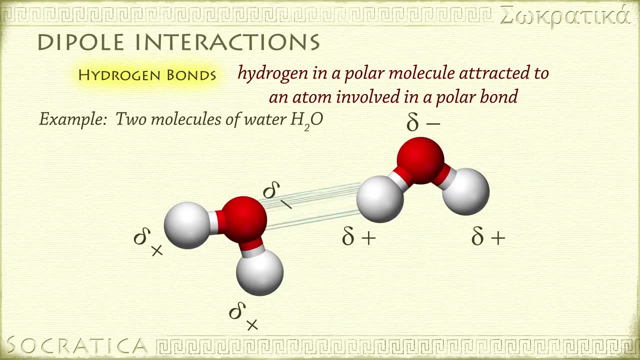 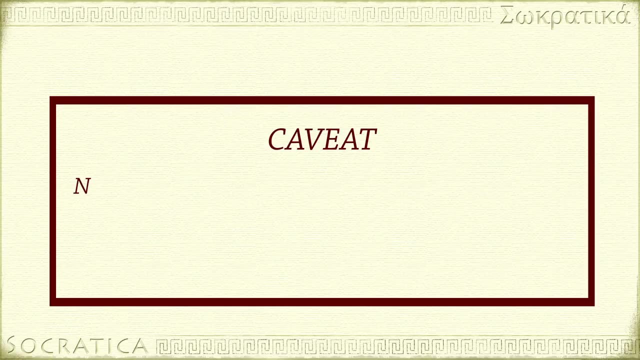 closer to themselves, resulting in a partial negative charge. The hydrogen then has a partial positive charge, so the two atoms in the different molecules are attracted to each other. Now here's a caveat, an exception, something to keep in mind. Not every hydrogen bond. 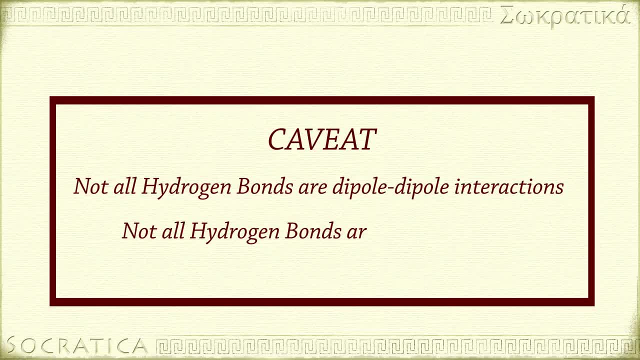 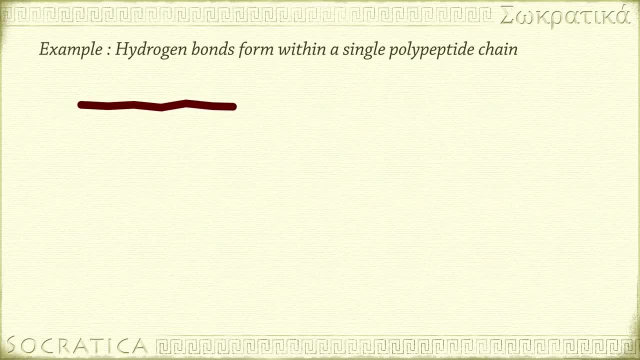 is a dipole-dipole interaction or even an intermolecular bond. There are cases of hydrogen bonds within a single molecule. For instance, if you study biochemistry, you'll learn about how hydrogen bonds are formed within a single polypeptide chain. 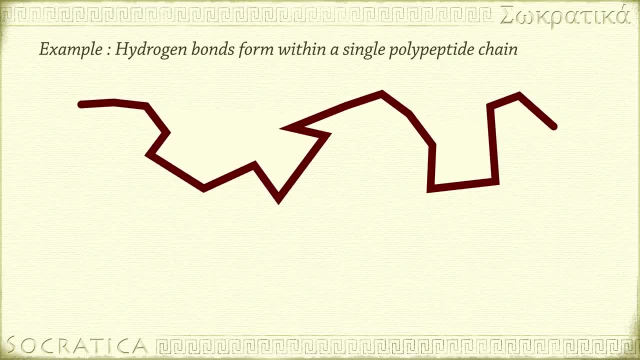 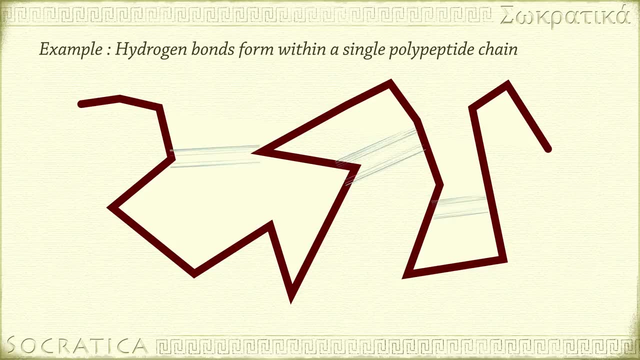 that is a string of amino acids as it folds up to form a protein. So that's a case of hydrogen bonds forming between different parts of the same molecule, But in chemistry you're almost always talking about intermolecular hydrogen bonds. 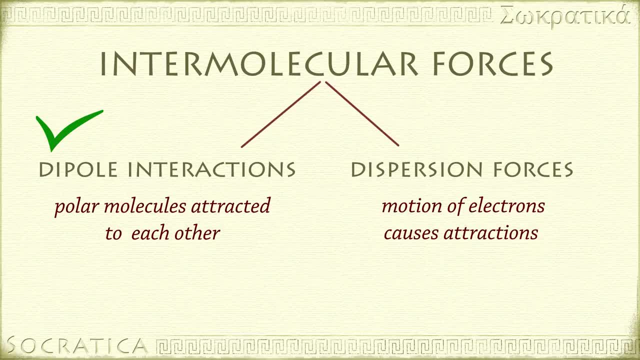 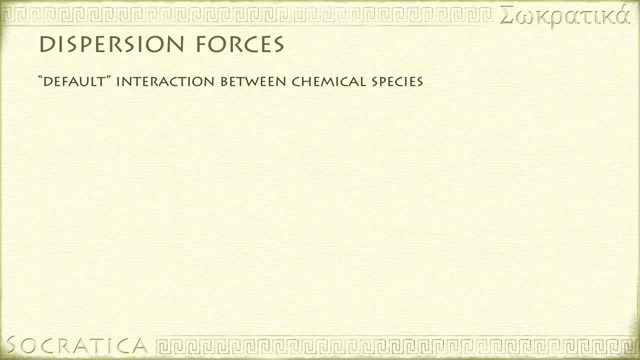 Now we've done a survey of dipole interactions. Let's move on to dispersion forces. You can think of the dispersion force as kind of the default interaction between chemical species. It involves the motion of electrons Since absolutely every atom and every molecule. 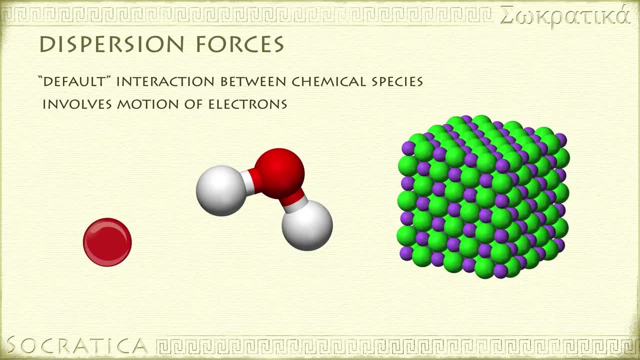 and every compound has electrons. every single kind of chemical species is going to experience dispersion forces. Thinking about the word dispersion, you'll see that the dispersion force is the key to remembering this force. How are the electrons dispersed or distributed in the cloud around the chemical species? 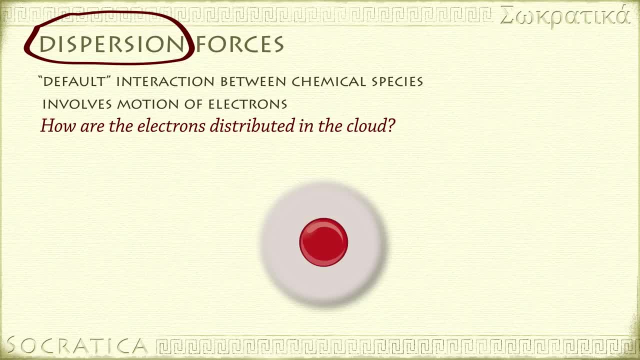 Are they absolutely evenly distributed? Yes, they could be some of the time, But a lot of the time, in fact almost all of the time, there will be an uneven distribution of electrons on the very, very surface of any given molecule. Think of it like patchiness. There will. for a brief, 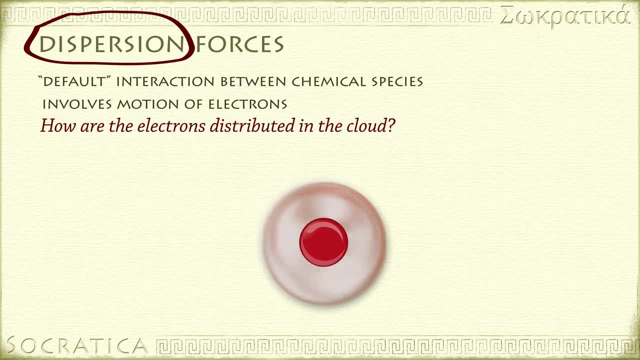 moment be a patch that is more negative than another patch. One patch will be more positive than another patch In the next moment because electrons are constantly in motion. the patch is gone. There will be a different kind of patchiness, Because this is true of all chemical species, every molecule, every compound, every atom. 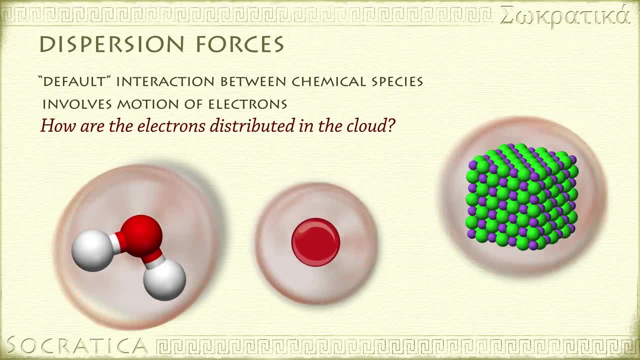 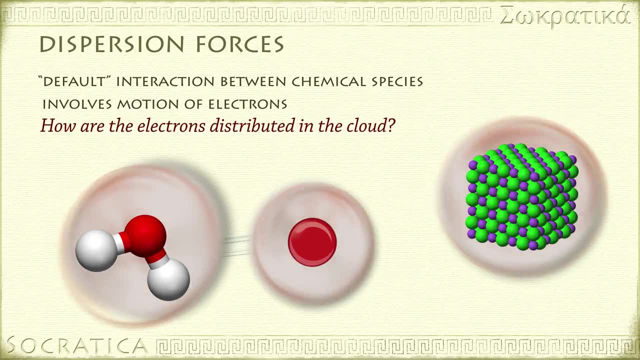 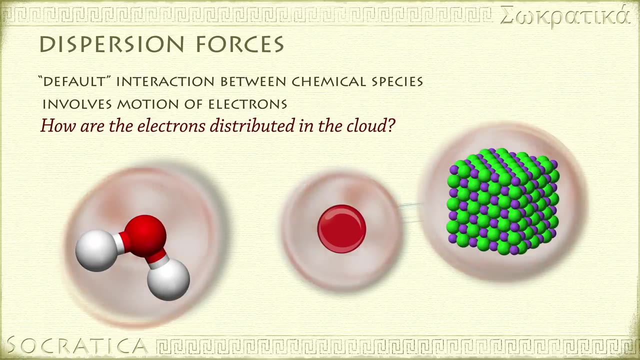 there will be some degree of attraction due to this kind of patchiness. For the briefest of moments, a negative patch on one molecule will line up with a positive patch on another molecule. Then, in the next instant, these patches have disappeared, or rather redistributed. 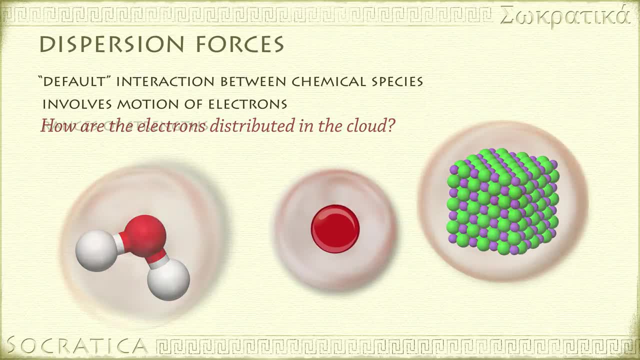 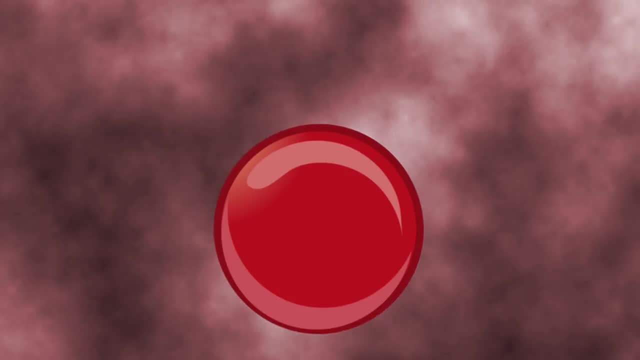 Imagine these bonds blinking on and off at a dizzying speed. There are ranges of strengths of dispersion forces. The larger the molecule, the bigger the electron cloud, the farther the electrons are from the nuclei, and so they're held less tightly and so they can move around. 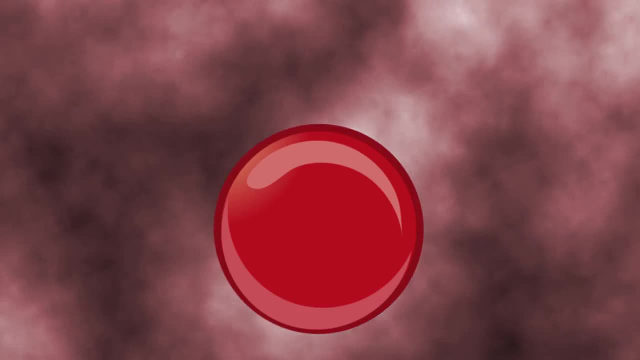 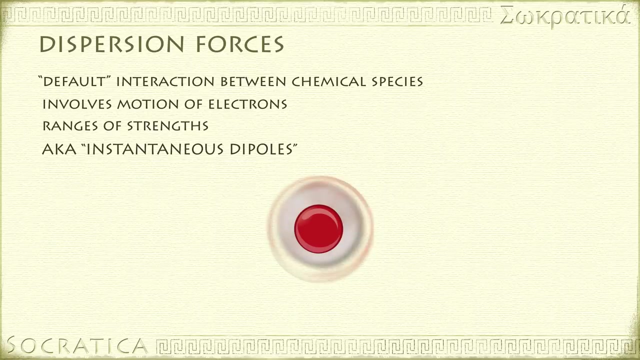 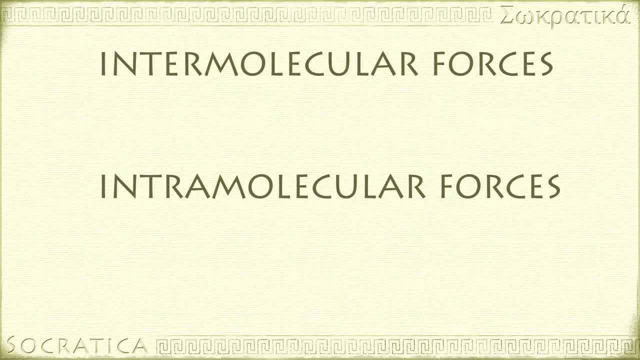 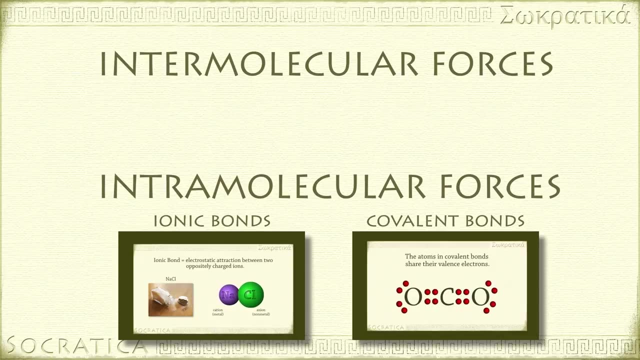 Careful you don't confuse intramolecular bonds with intermolecular bonds. In previous videos we discussed intramolecular bonds, the strong bonds that hold individual compounds together, ionic bonds and covalent bonds. Intra- refers to the bond between electrons and yêu. равно- refers to the bond between electrons. 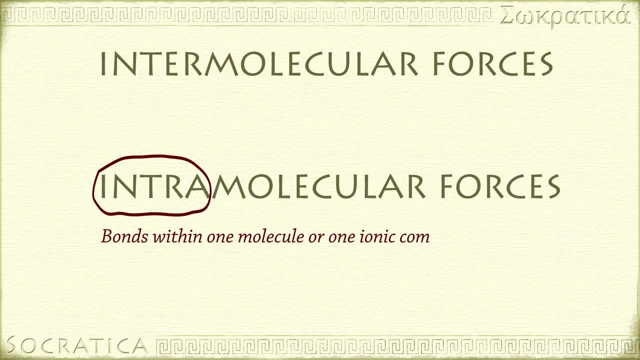 so that's the strength and the strength and the elasticity of the bonds, And this is the value of intermolecular bonds to the bonds within one molecule or one ionic compound. Inter refers to the bonds between two different chemical species, Intramolecular forces, the forces that hold one compound together. 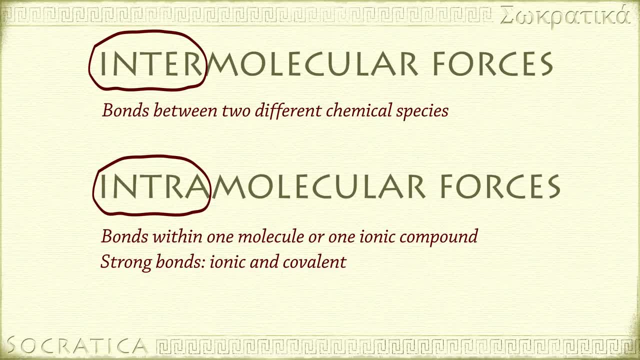 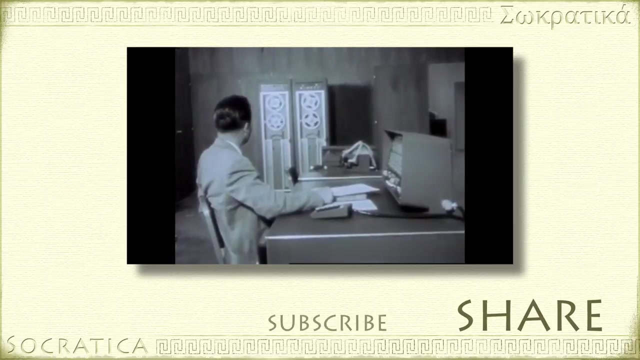 are much stronger than intermolecular forces, the forces between different molecules. Intermolecular forces are all essentially electrostatic interactions, attractions between positive and negative charges, just far weaker than the strong electrostatic attractions involved in ionic bonds. If you found this video helpful, share it with your friends and don't forget to. 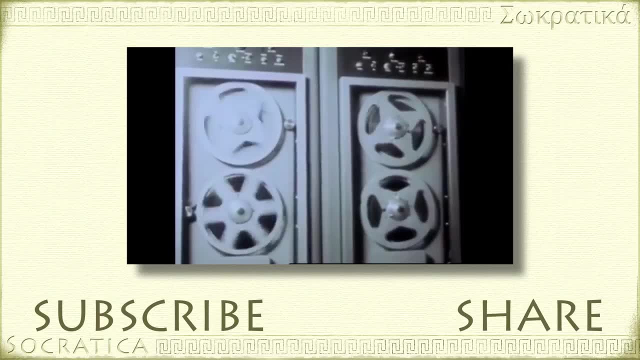 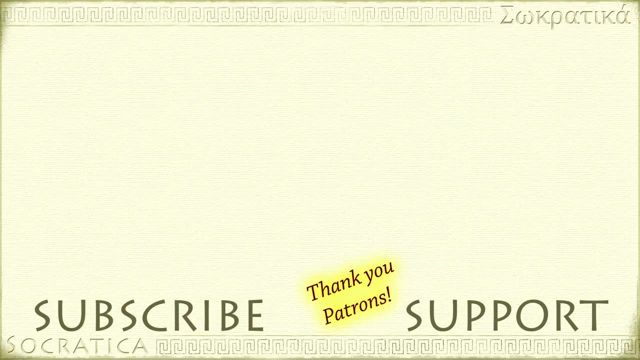 subscribe so you'll hear about our next video as soon as it comes out. If you'd like to support our work and help us get out videos faster, you can become our patron on Patreon. Every bit helps. Thanks for watching Socratica. you.